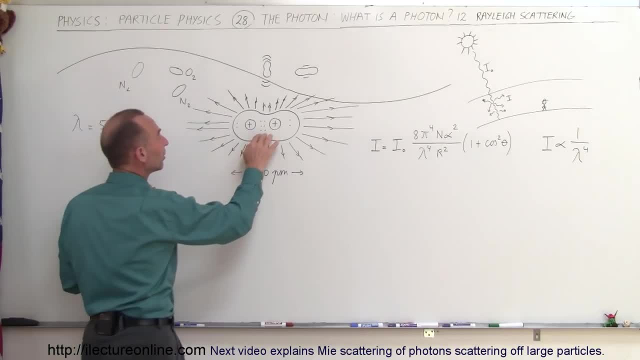 them, which must be shared in a valence, in a sharing relationship. And then we have two additional electrons which can be in the outer orbitals of the individual atoms, forming a molecule. like that, It turns out that this molecule is symmetric in all respects. so 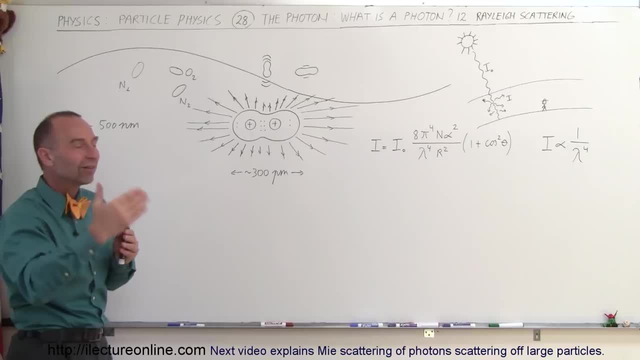 that the charges are symmetrically divided over. so there's no one side that's more positive and the other side that's more negatively charged, so there's an equal charge distribution in the molecules, perfectly symmetric. Same with oxygen, except with oxygen we have four. 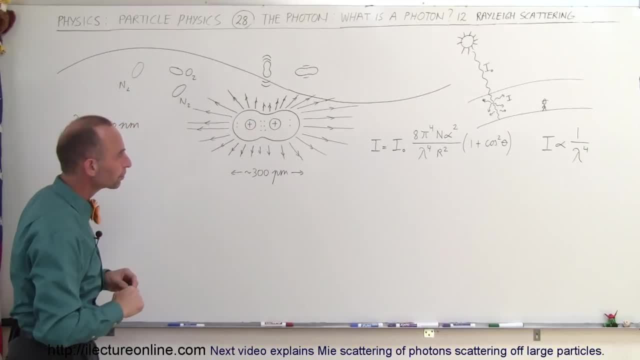 valence electrons here and only four being shared between the two, But the principle is the same, and so it turns out that these molecules can actually vibrate. They vibrate in various directions, so the molecule can vibrate. like this, it can vibrate. 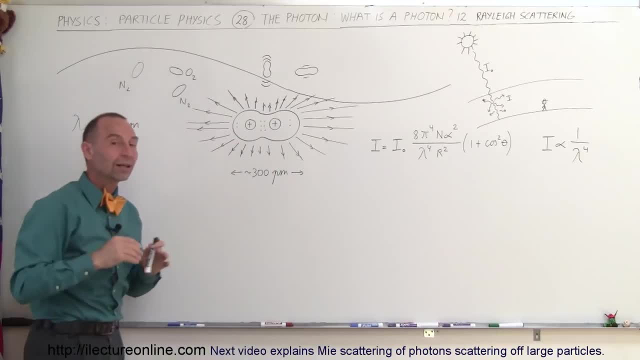 like this, but it's more likely to vibrate like this. And so when an electromagnetic wave or a photon comes along- and of course a photon- what does it do? It changes the electromagnetic field around these air particles, the air molecules, for example, and it causes 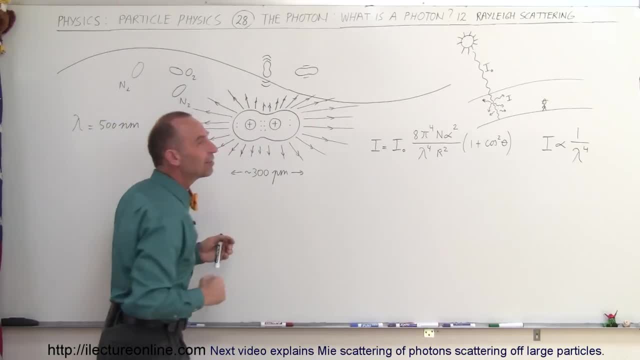 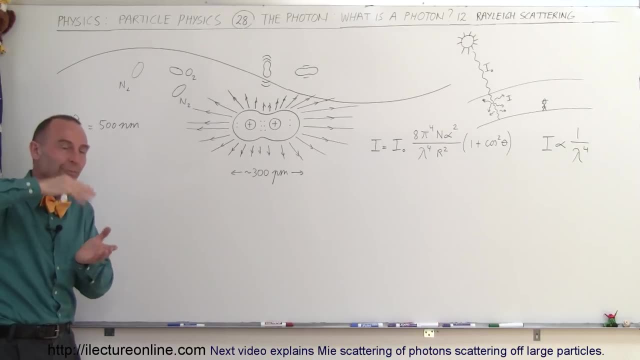 them to vibrate at the same frequency as the vibration of the electromagnetic radiation or the vibration of the photons, Which means that as the photon vibrates, the electrons come through and they vibrate. the change in the electromagnetic field will cause the molecules in the air to vibrate as well at the very same frequency. Now they're more. 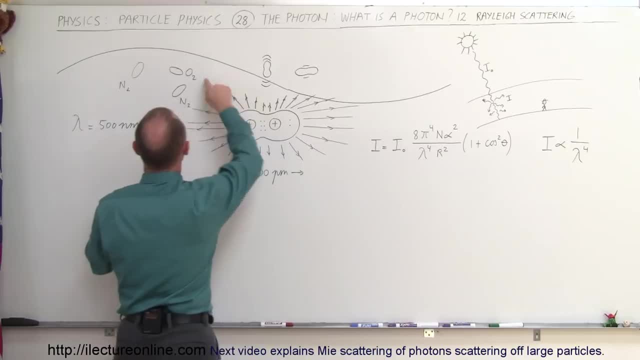 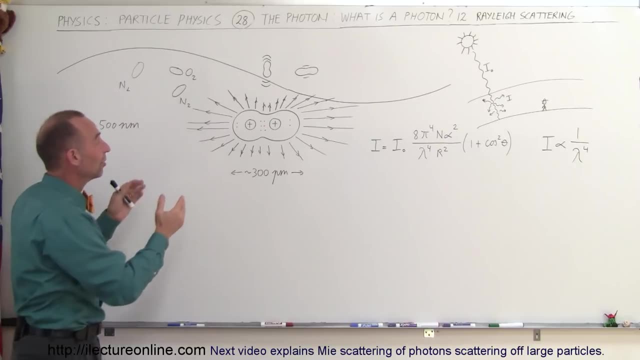 likely to absorb the energy in this direction than this direction. and since the molecules have all kinds of different orientations, you will then find that the scattered light, because what happens is a molecule will absorb the energy and then re-emit the energy without 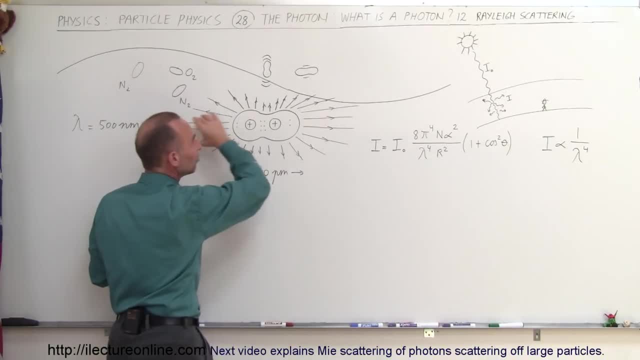 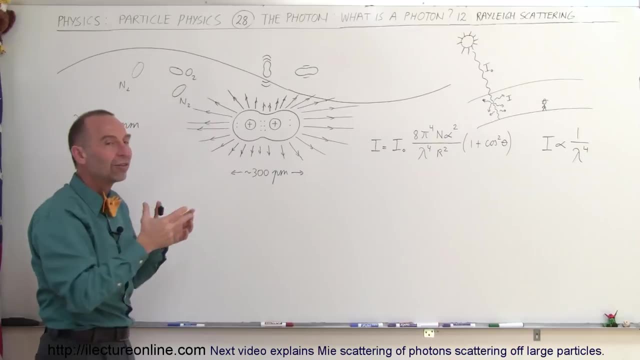 any loss, but it'll transmit the energy in this direction more readily than in this direction, and because of that we tend- the air tends- to polarize the scattered sunlight and so there's a certain polarization factor to it. But because of that, because 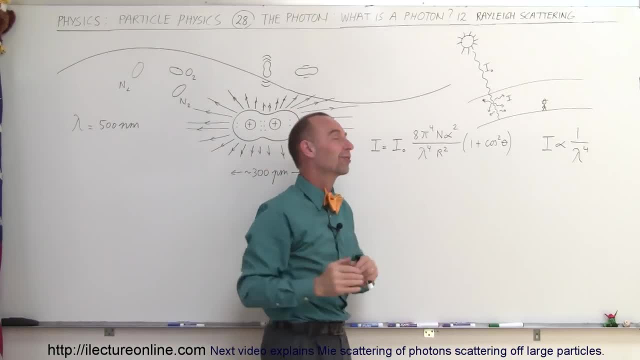 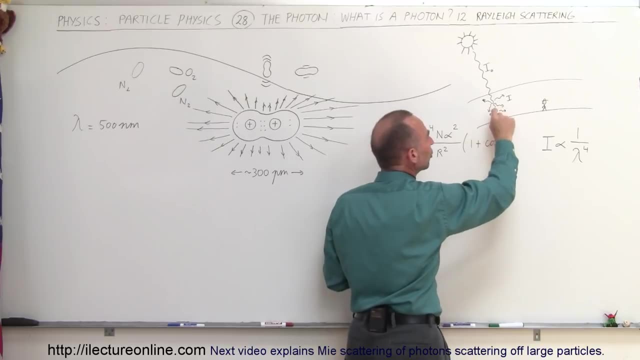 of the different orientation. here I have a little picture of it, a primitive picture, I may add. so you have the sunlight coming in from the sun. it enters the atmosphere and as it starts hitting these air molecules it begins to scatter out, but more so in one. 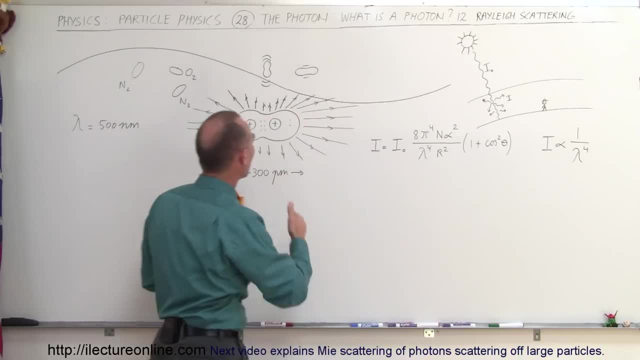 direction versus other directions, so the light tends to get polarized relative to the direction of the light, And so that's what we're going to talk about today. We're going to talk about the wavelength of the incoming sunlight. Because of that, 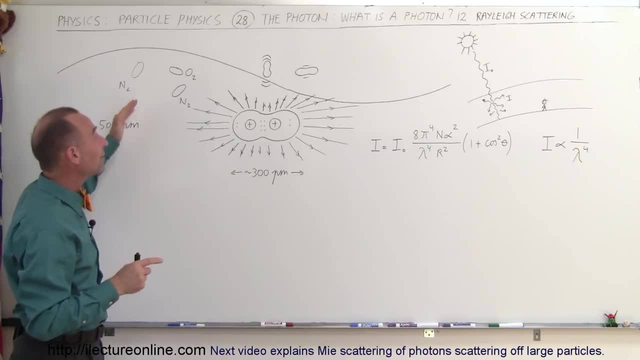 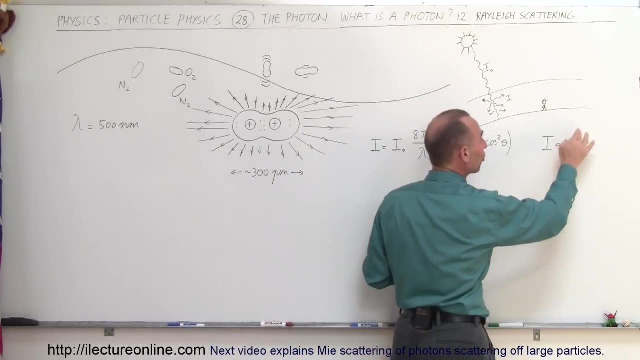 and also what we find is that the amount of scattering depends on the wavelength of the incoming light. It turns out that the intensity of the scattering, the amount of light that gets scattered, is proportional to one over the wavelength to the fourth power. It's 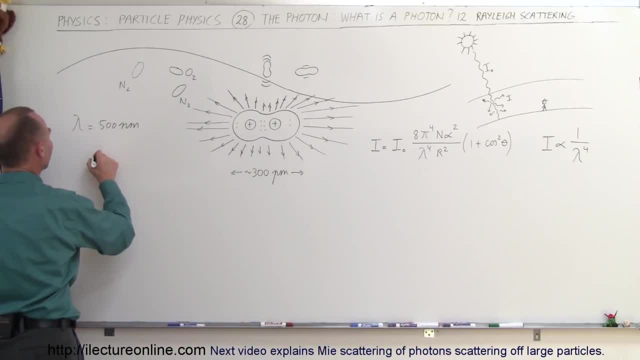 kind of interesting. Let's explore that for a moment. So we know that the wavelength of sunlight ranges anywhere from 400 nanometers for the purple light to about 700 nanometers for the red light. So this is for red light and this is for purple light. So which light? 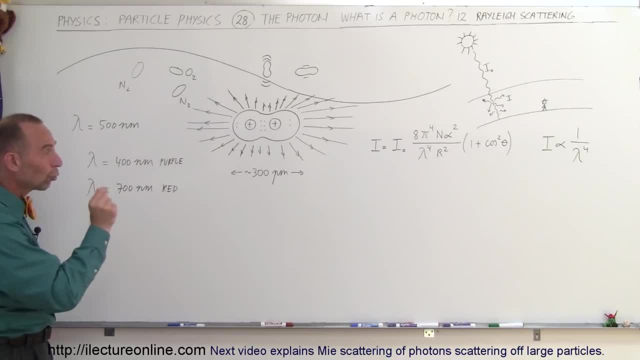 gets scattered more Well. it turns out that the shorter the wavelengths, the greater the scattering. the longer the wavelengths, the less the scattering. So it turns out that if there's a higher frequency photon with a shorter wavelength, it's more likely to 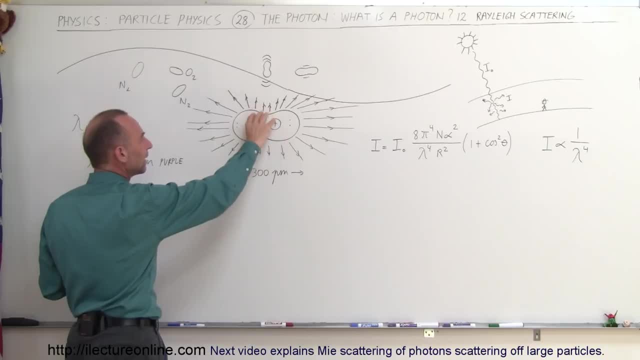 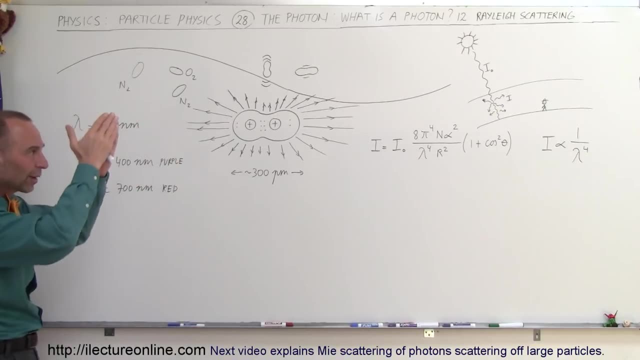 interact with the air molecules, with the nitrogen and oxygen, more likely to distribute its energy into those molecules and get it re-radiated out, so that the light no longer comes directly towards the observer, but that it's scattered in different directions, Part of the reason why the sky 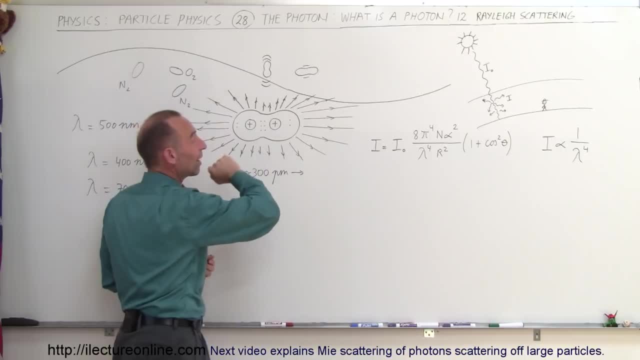 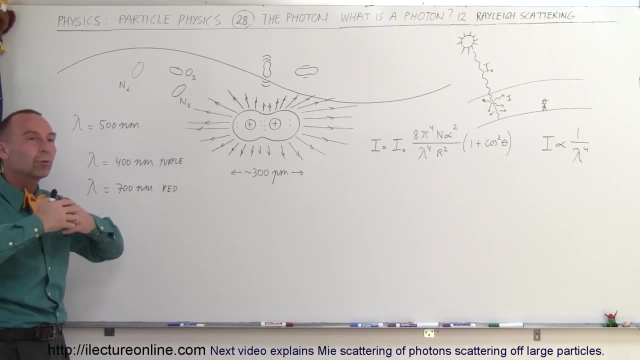 is blue is because blue is more likely scattered in this fashion because it has shorter wavelengths. Shorter wavelengths means higher intensity of scattering, And so therefore the sky looks blue because blue light tends to get scattered out way more than red light. The reason why 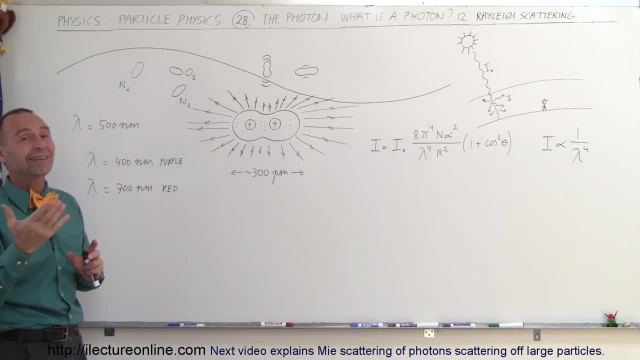 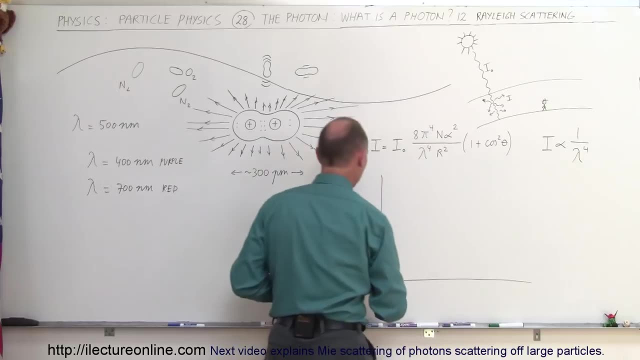 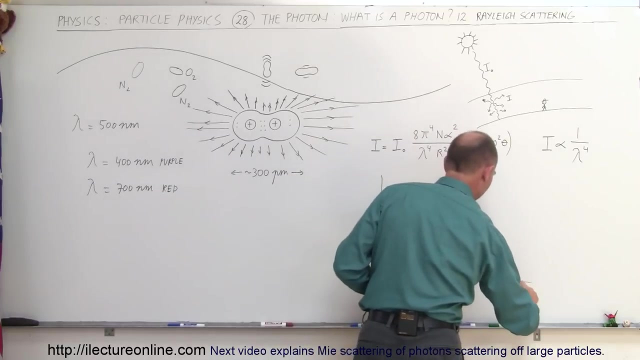 the sky doesn't look deep. dark blue is because all of the wavelengths get scattered as well, but not quite to the same quantity. If you draw a little chart of that and so you say this is blue light at 400 nanometers or purple light at 400 nanometers and this is red light at 700 nanometers, the amount: 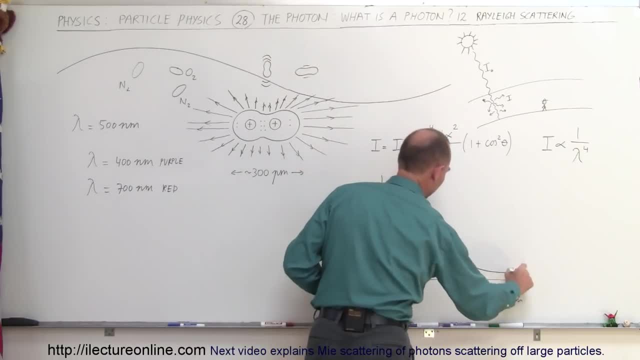 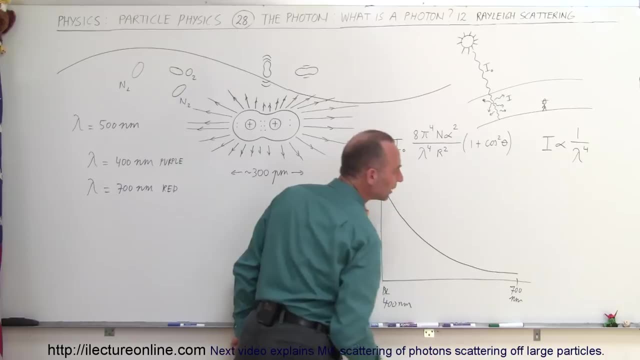 of light getting scattered out will vary like that according to wavelength. A much greater proportion of blue light gets scattered out, and very, very few of the red photons get scattered out in comparison, Ratio-wise, let's take a look for a moment. 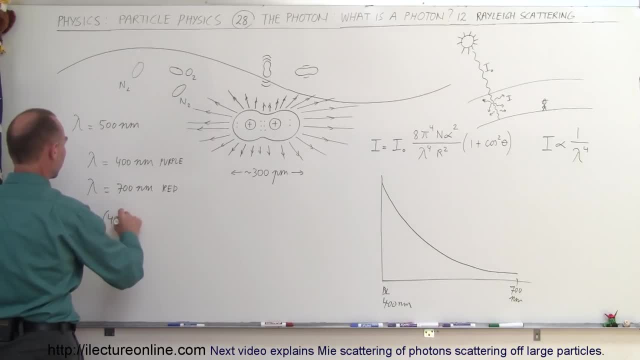 Let's say that we take 400 to the fourth power and we take 700 to the fourth power, and then we'll take that ratio and see what we get. Actually, we don't have to do 400. We can go four by itself and get rid of zeros, because we just want to care about the ratio. 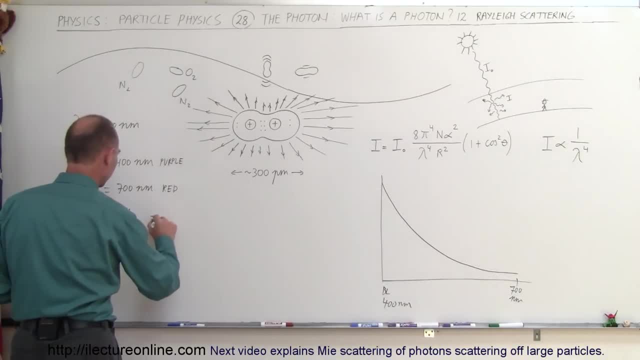 So four to the fourth power is 256.. Seven to the fourth power is 2,401.. So, ratio-wise, how much more the blue light gets scattered out compared to the red light if we take the 2,401, because it's inversely proportional. so we have to take the inverse of that. So 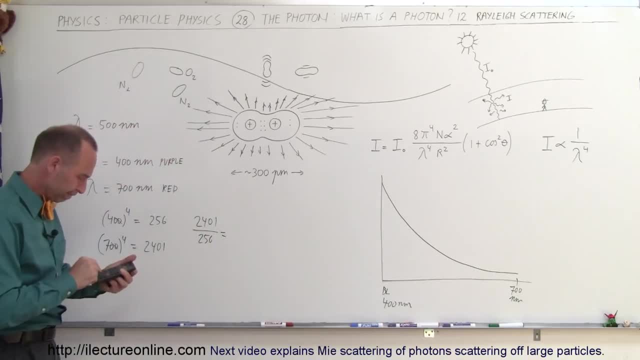 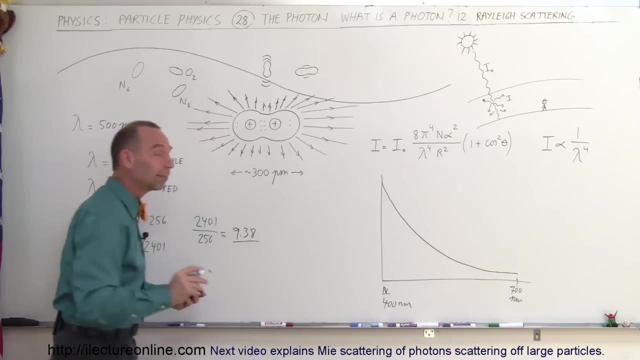 2,401 divided by 256, what do we get? We get 9.38, 9.38, which means that blue light is more than nine times as likely to get scattered out in the atmosphere as red light. so ratio of about nine to one, Now part of the reason. 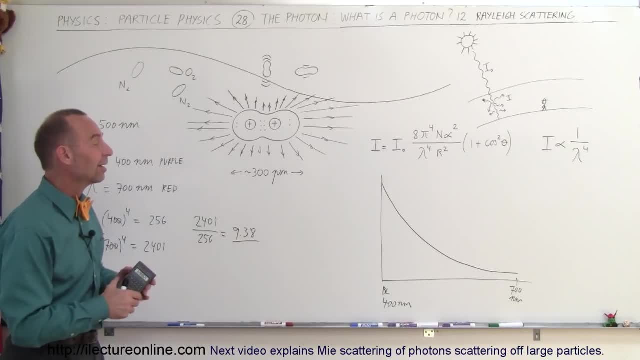 why not nine times as many blue light gets scattered out in the atmosphere? is because the blue photons get scattered out. is because the distribution of light coming to the Earth doesn't have as much blue light as it has more of the yellow, green and orange light. 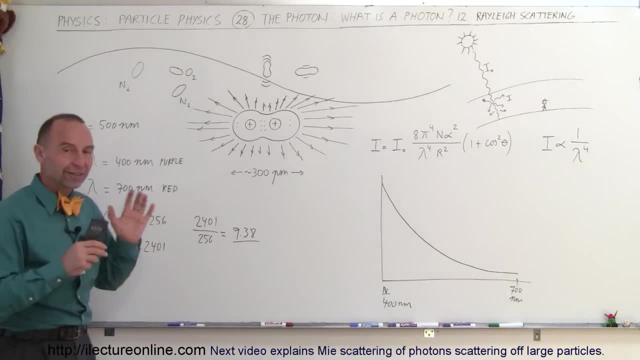 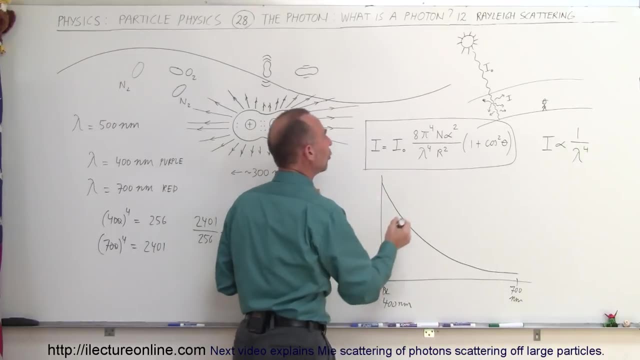 Anyway. so to get a feel for the Rayleigh scattering, let's take a look at the equation right here. This is the equation that defines the Rayleigh scattering. Notice the one over lambda to the fourth factor in there. Also notice that it depends on the number of molecules. 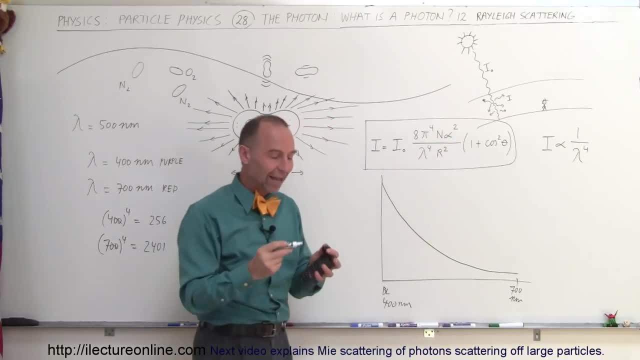 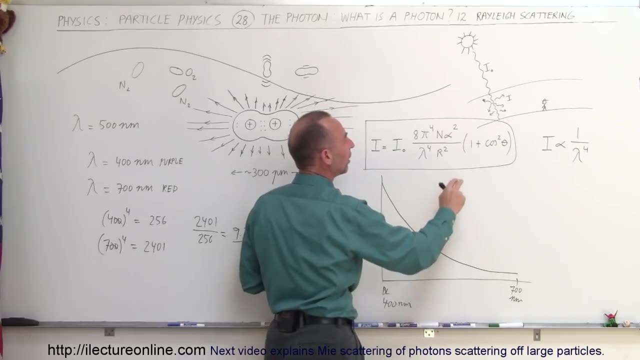 in the air, of course, and how effective those molecules are in the atmosphere. So we're going to look at how effective those molecules are at reflecting or scattering the light. So different molecules have a different proportion in which they can scatter the light. Also. 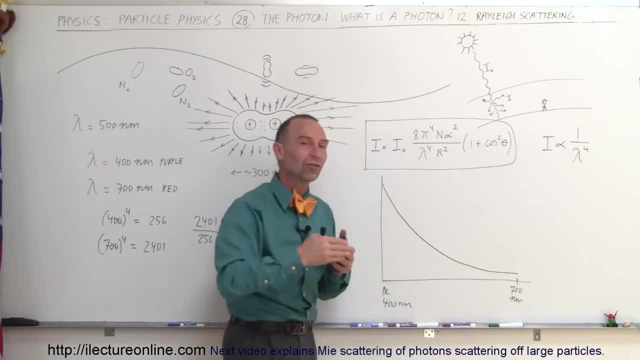 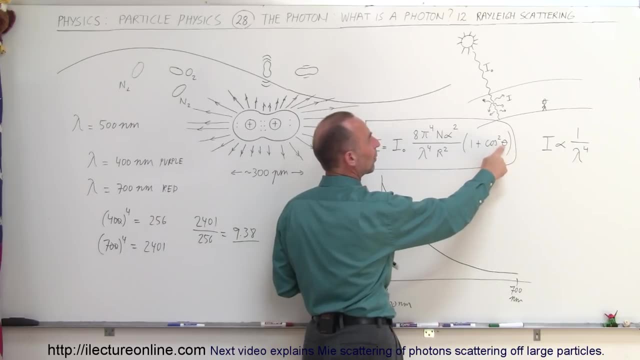 of course, the intensity is proportional to one over the distance squared. As you go farther away from the source, you get less and less of the intensity. And finally we have the scattering angle, theta- right here. Notice that when theta is equal to 90 degrees, the 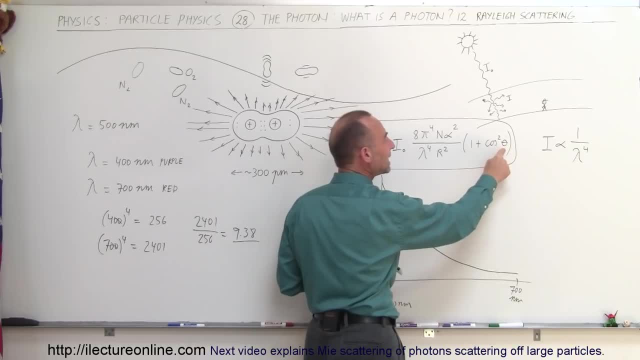 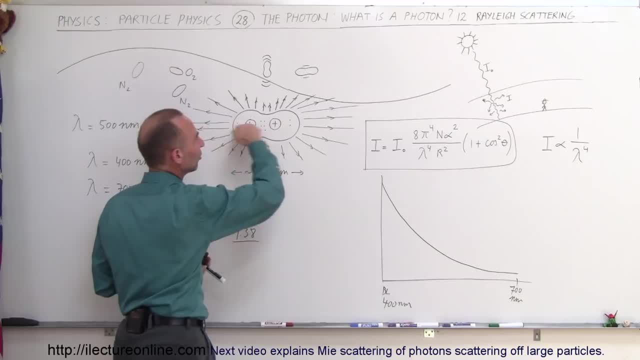 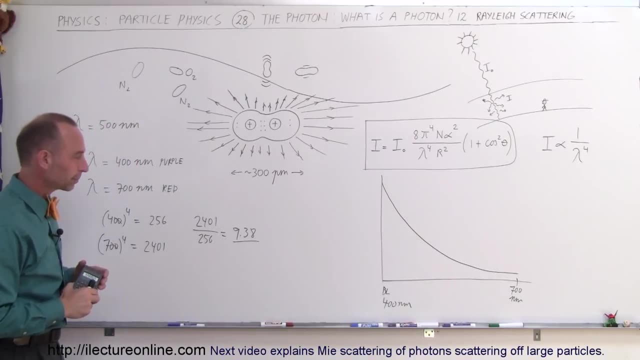 you get one plus one equals one equals two, which means that the scattering in this direction is about twice as much as the scattering in this direction, And so that's, by definition, Rayleigh scattering. Again, understanding a photon is understanding how it interacts with matter. Here we have a photon that has a wavelength that's over a thousand times. 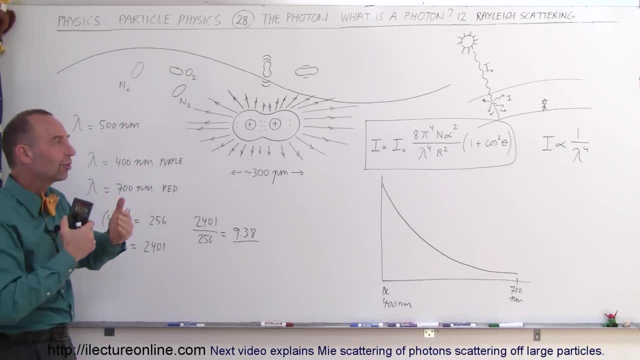 the size of an air molecule. yet there's the interaction because of the changing electromagnetic field that causes a scattering to take place And hopefully that again gives us another window into the look of what the scattering is. Rayleigh scattering Again. understanding a photon is understanding how it interacts.